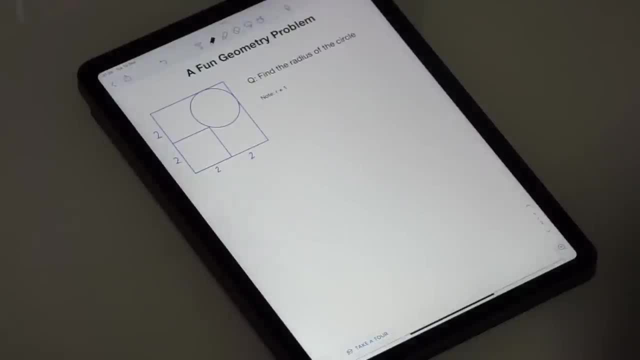 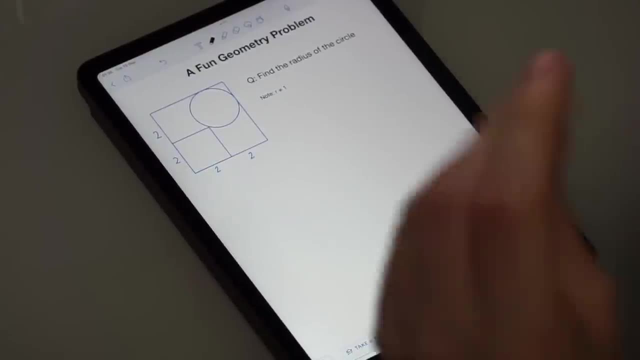 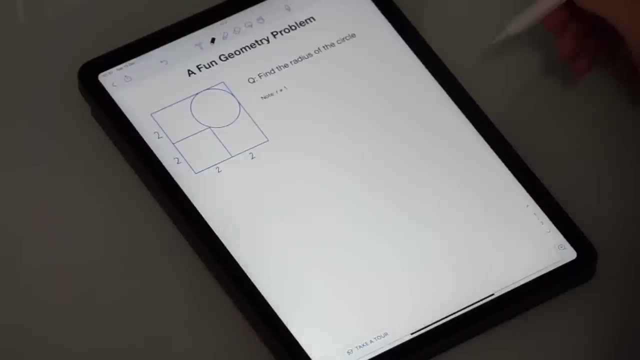 hey, everybody, everybody, everybody, everybody, everybody, everybody打 Scorpio. How's it going, everybody? And welcome back to another ASMR MRMAPS video. In tonight's video I have just a fun little problem that I thought I would solve with you all. 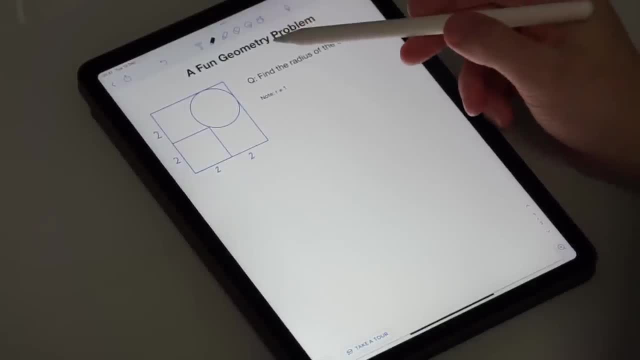 and it is a geometry problem, as you can all see. No, this is a problem that I actually first saw on TikTok a few months back, and it fascinated me and I thought I would try and solve it without looking at the tutorial. so I gave it a go and I actually managed to do it. 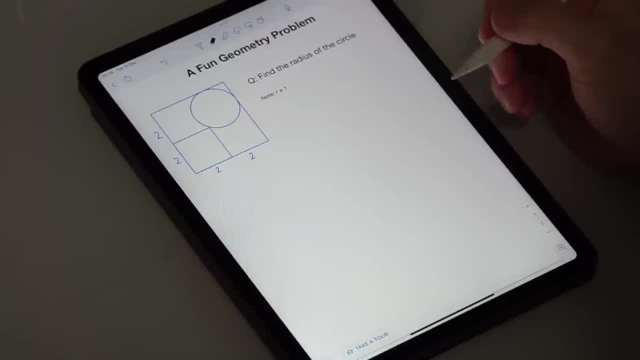 correctly and I thought I would share it with you all. show you all the solution, talk through it with you and well, first and foremost, if you all want to give it a go before I talk through the problem with you, then feel free to pause, try and give it a go. 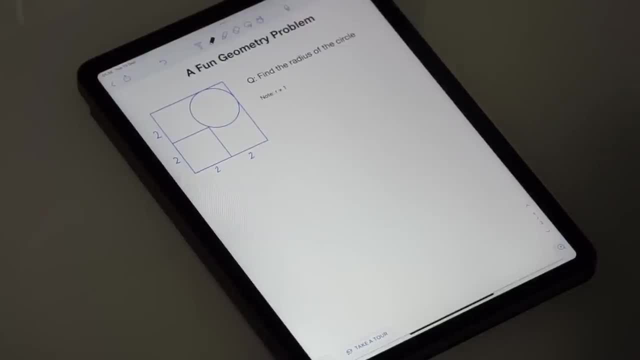 but to quickly sort of explain the problem to you all, first we have this square, with inside we have another square and a circle which you can see meet at this little point right here, and we have some dimensions around. note that that is 2 and 2, not 22. 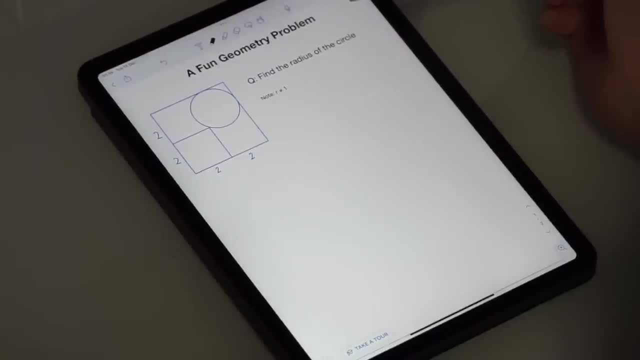 and the question is to find the radius of the circle. and we have a little thing here that says: note that the radius does not equal 1, so it's not like it's half of this 2, so feel free to give this problem a try yourself. 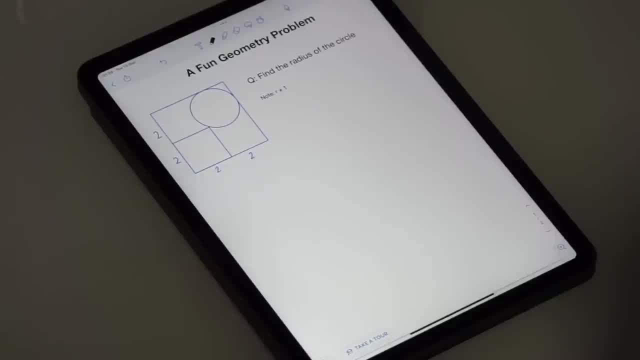 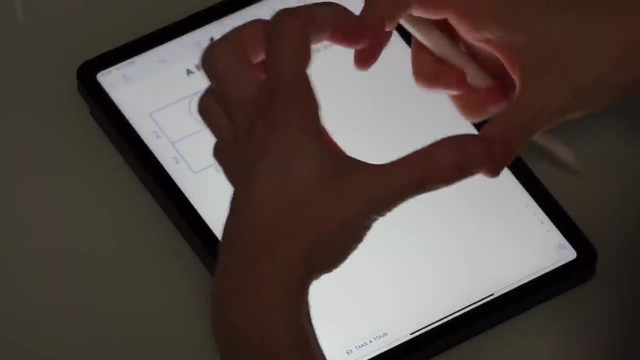 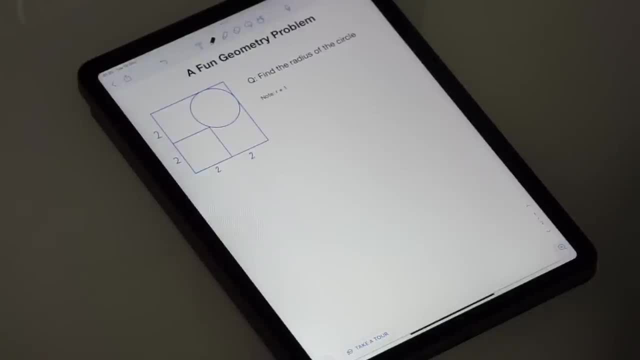 a lot of tips and improvement things from the last video I saw in the comments, a lot of which I'm going to try and implement in this video and future videos as well. these videos are quite tricky to actually get a good camera angle, so I'm going to be testing out a lot of different things. 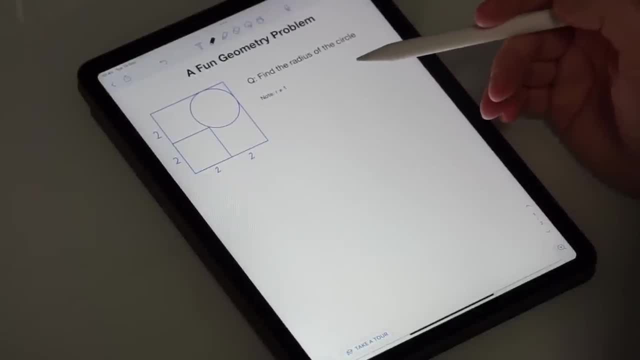 a lot of different backgrounds as well, and a lot of different things. other videos might not always be on the iPad, it might be on paper, it might be on my PC, it might be on a whiteboard, and so on and so forth. but anyways, without further ado, 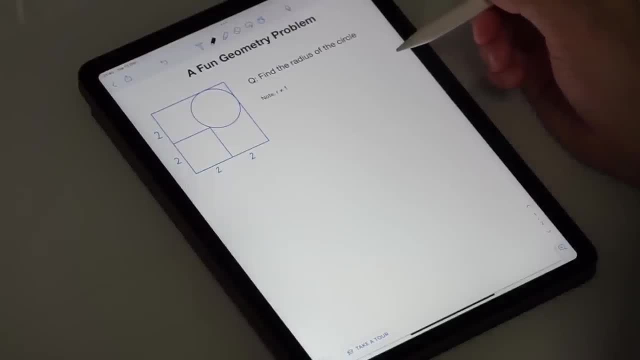 let's get into this problem and actually get into how I tackled this problem. so again, we have this square which measures 4 by 4. you can see, from the midpoint of the squares, lengths or edges is 2. so therefore, that's how it's: 4 by 4. 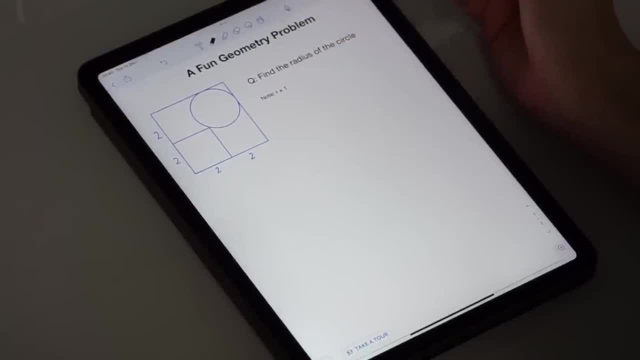 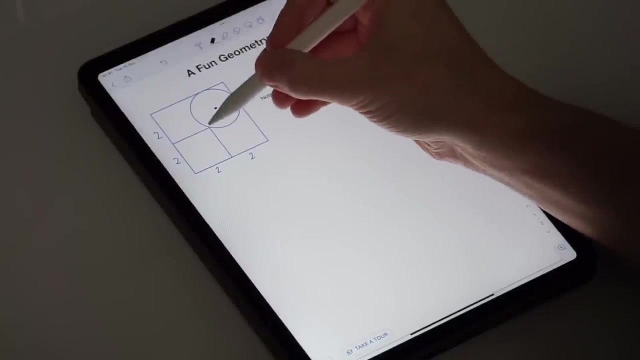 so if we want to work out the radius of the circle, well, let's first and foremost put a little centre point on this circle, because when I first went to go and tackle this problem, I figured: ok, well, we can see that the radius is simply just from here to here. 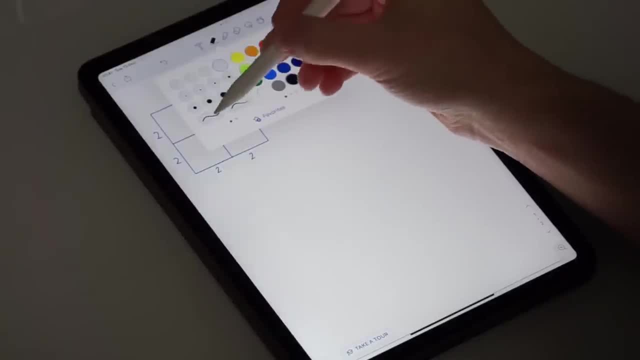 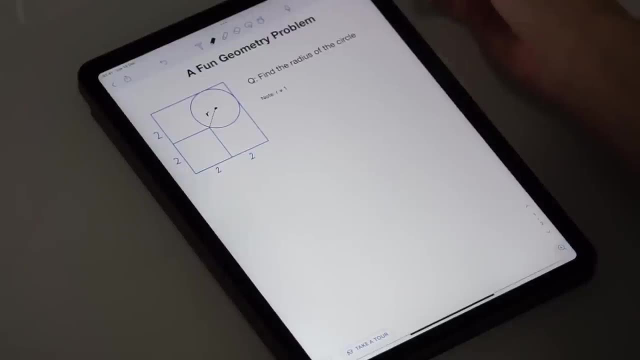 right, we can call that. let's call it R. so I thought: well, it's just going to be one, because it's the same as what it is from here to here. as you all know, the radius of a circle is from its centre point to the edge of the circle. 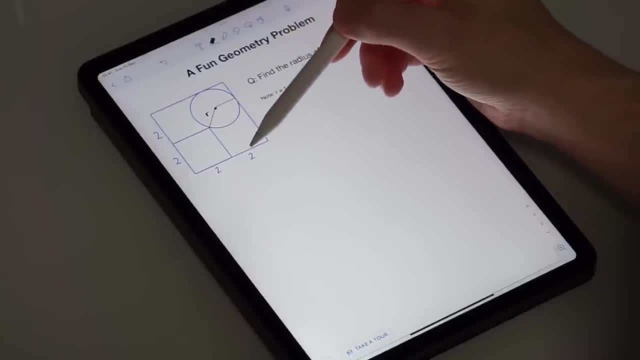 and I thought: well, that looks like one because it's halfway between the middle, but it's not. we were told that in the question, so it cannot be one. so we have that. this is R, in fact. I'm actually going to just draw the radius back out here. 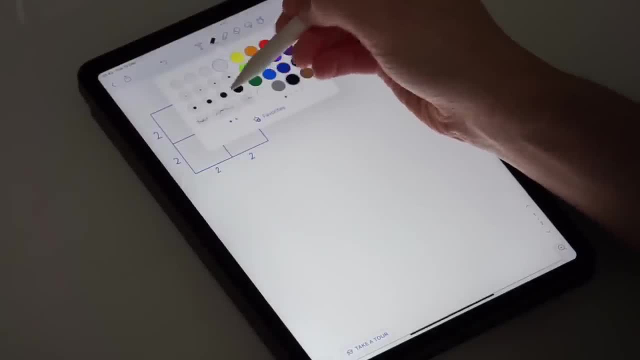 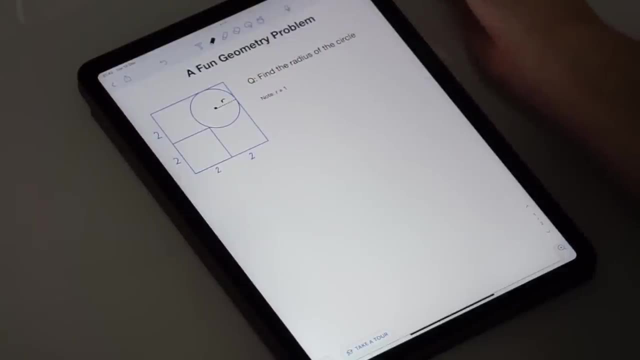 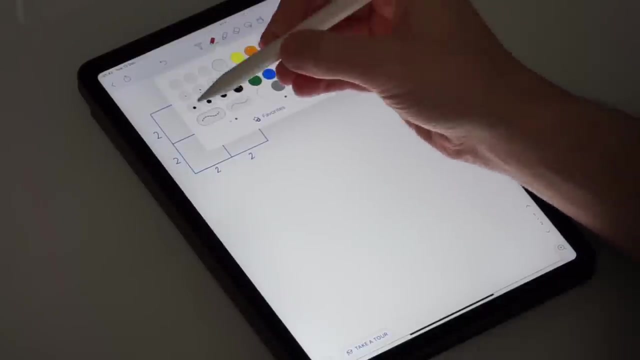 I think for later it will be a bit more useful if I just leave it like this. so what do we know? well, we know that the square is 4 by 4. thus, if we take, let's say, a nice red, a dotted line, a dotted line. 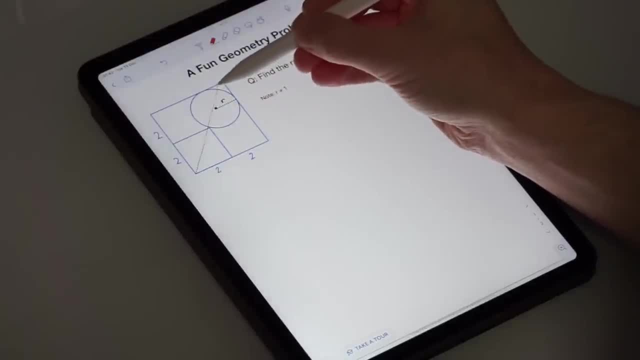 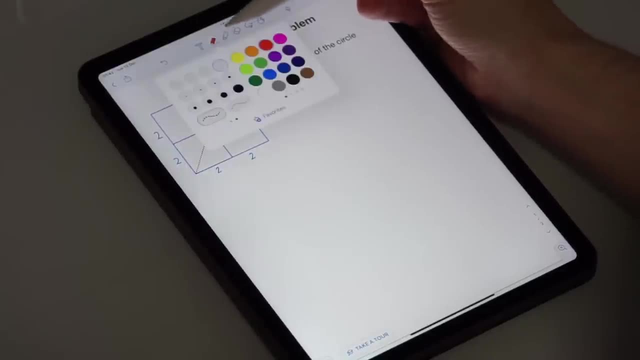 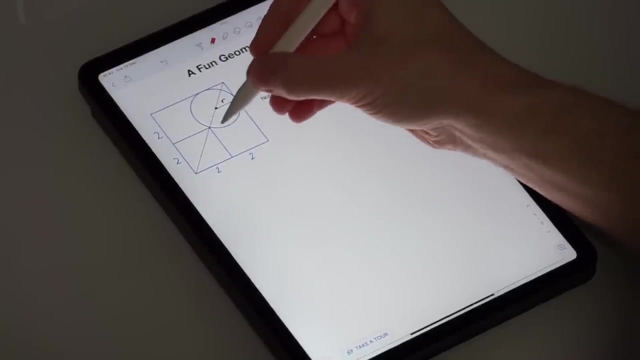 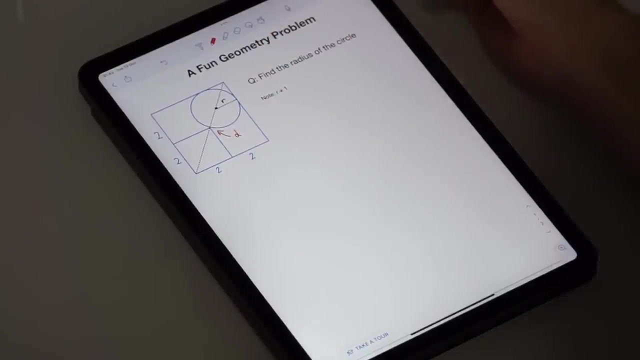 from one corner of the square right to the other corner. we can call this the diagonal of the square. I am going to just for this video, we're just going to call it. let's say, um D. now we can actually evaluate what D is using. do you know what it is we can use? 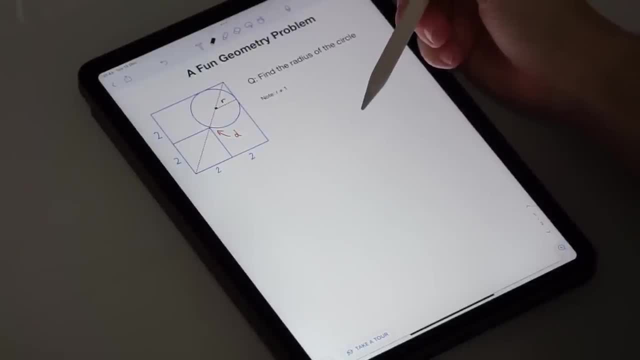 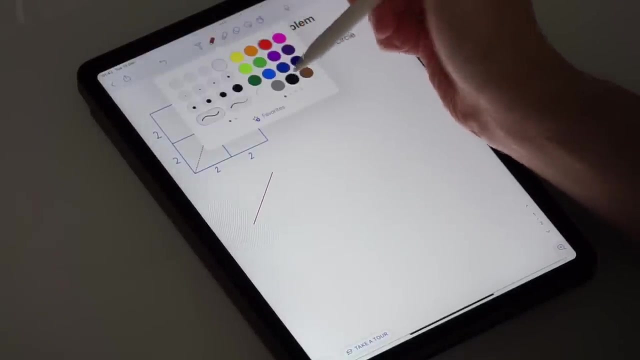 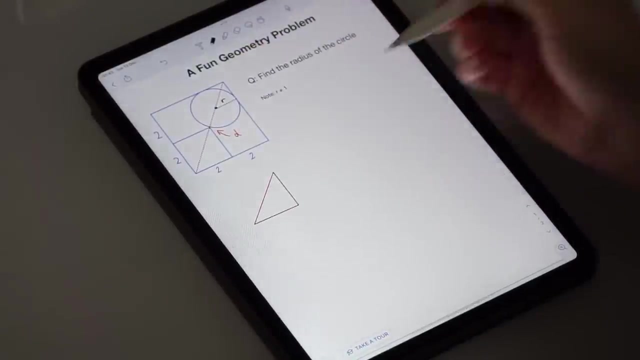 to work out what D is. I'll give you a little hint. if I take that line D- let's get this red back up- and if we connect this line up a little bit like this, a little bit like so, does this give you a little hint at how we can maybe work out? 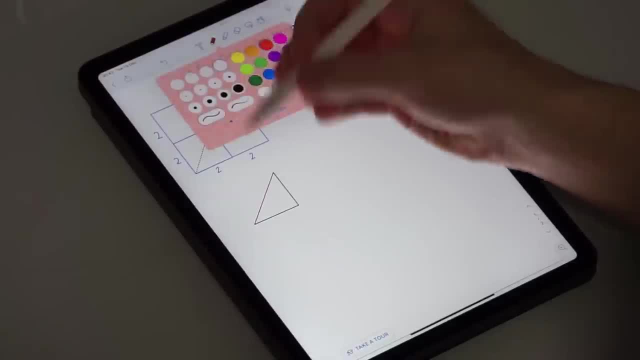 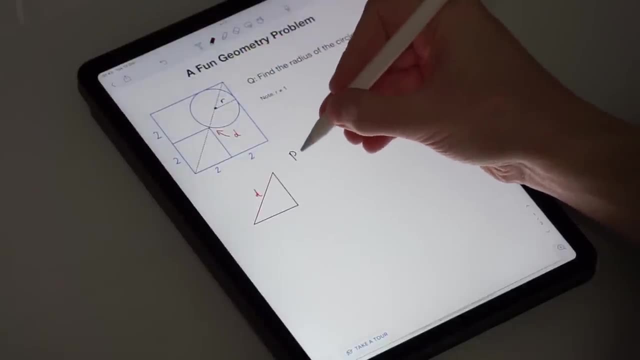 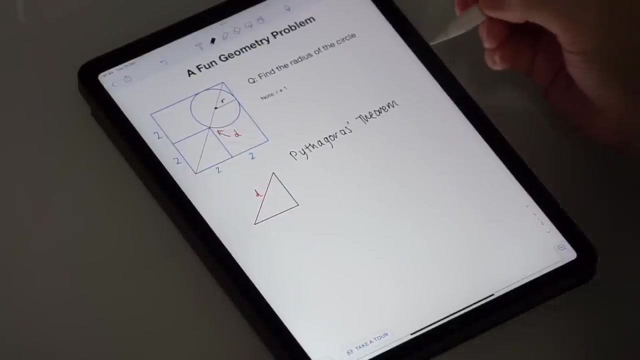 what D is. that is correct. we can use a little bit of Pythagoras's theorem to evaluate D. so how can we work out D? well, simply put, D is going to equal, or D squared is going to equal, the sum of the edges of this triangle. 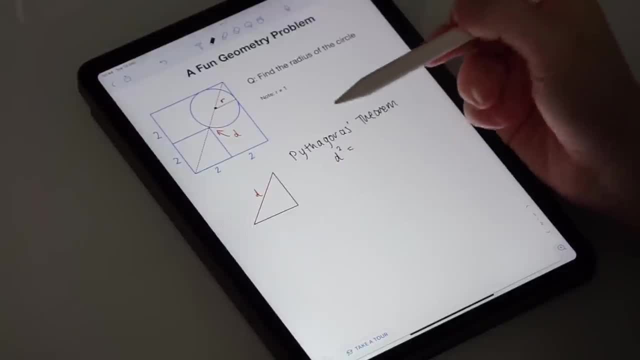 the adjacent edges, um, or the base and the height squared. now what are they in our case? well, we can see that it is going to be four and four, so four and four. so we have four squared plus four squared. now, four squared is sixteen plus another four squared. 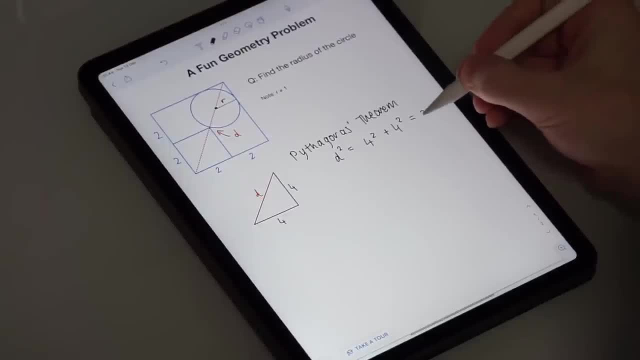 is thirty-two, so we can say that D squared is equal to thirty-two. therefore, D must equal the square root of thirty-two. now that's not like a nice um exact value, is it right? however, we can simplify, we can simplify, simplify. we can simplify this category. 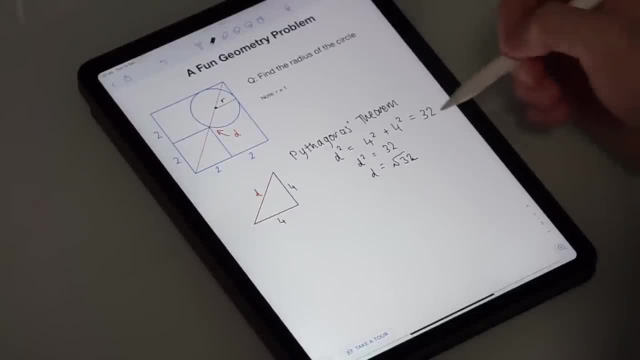 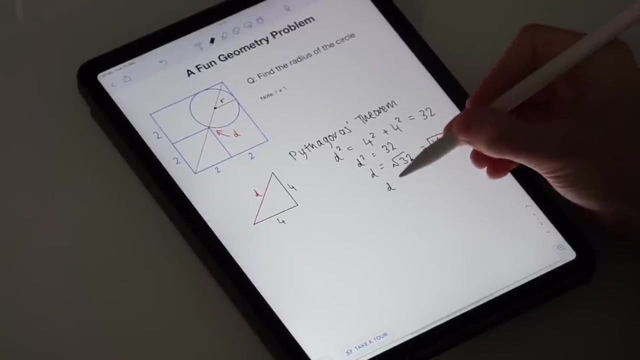 we can do a little bit of simplification. we know from CERT that we can simplify this CERT up a little bit, so let's do that. we can say that this is sixteen times two, like so, and when we simplify that even further, square root of sixteen is four. 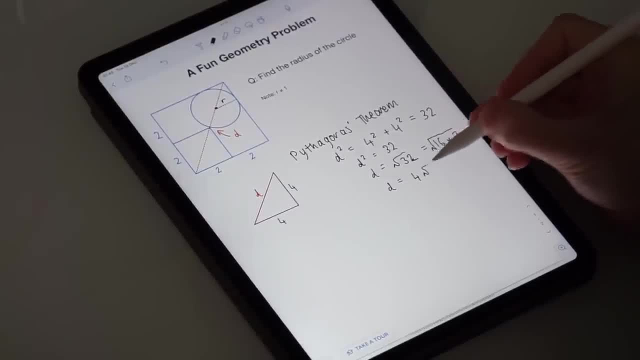 so we end up with: D is equal to four root two, and I'm gonna do a little bit of highlighting just so we can come back to this perhaps a little bit later on. um in the problem. so D is equal to the long diagonal is four root two. 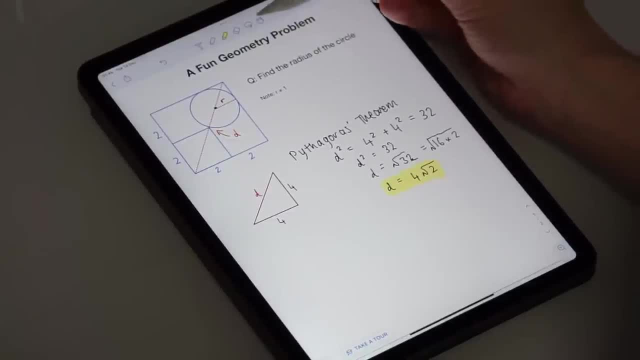 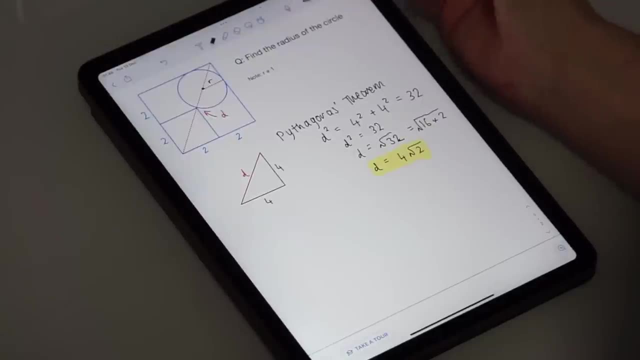 and we did that just with a little bit of Pythagoras. how easy was that? right? let's continue. let's continue on with the problem. so what else do we know? well, let's take a look if we have the diagonal D, if we can work out. 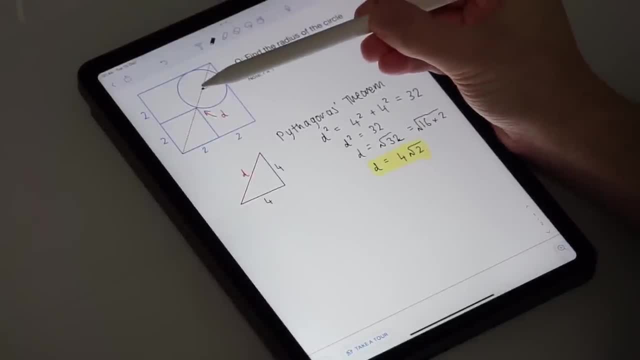 let's say this bit, this bit from here to here, and if we can also work out from this bit here to here, we can then in turn work out this value here which, as we showed right back at the start, is just the radius, because from the centre point of the circle 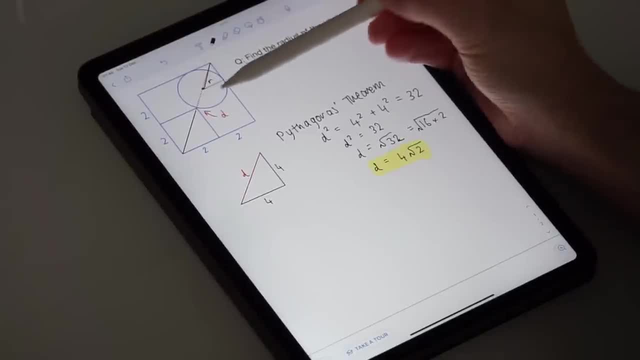 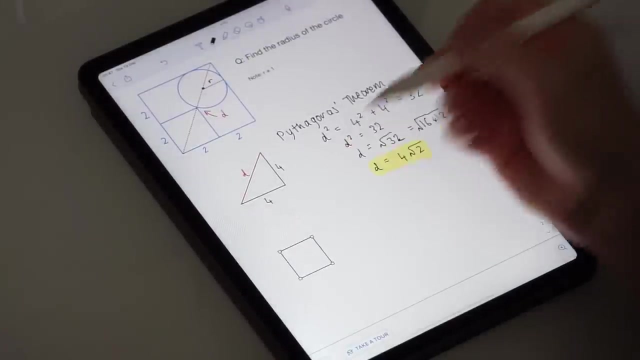 to any point. on its edge, on its um, circumference is just the radius. well, let's work out that line there and that line there. in fact, let's start with this smaller square. so let's draw out this little smaller square, shall we? there we go. that looks very good. 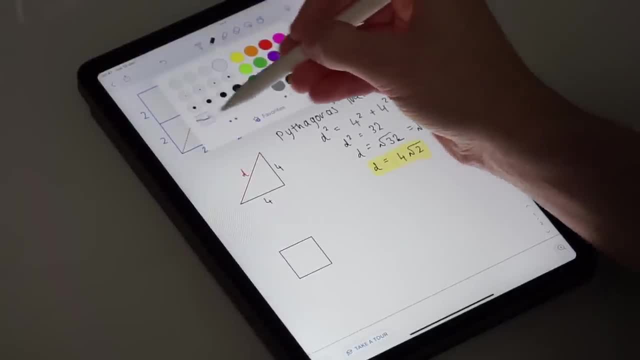 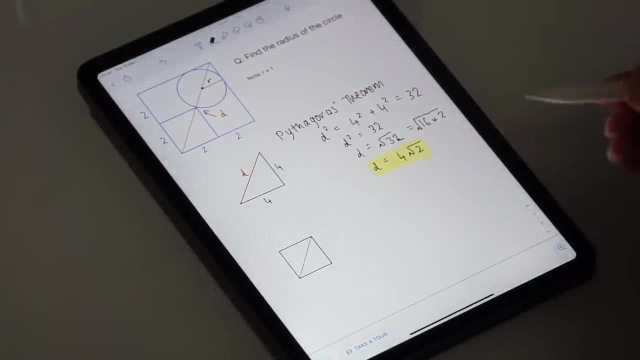 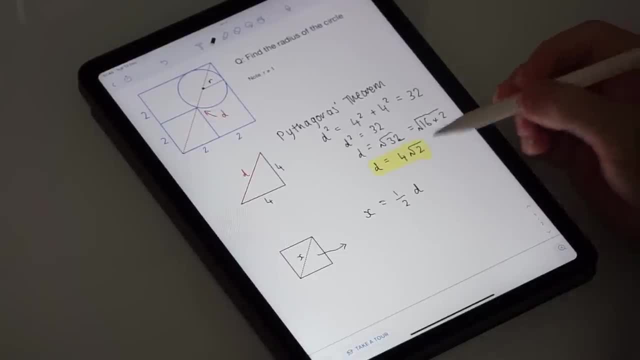 Now, what is a half d? Well, let's input our values. We have a half multiplied by 4 root 2.. And when we simplify up here, we get that x is equal to 2 root 2, because 4 times a half is simply 2.. 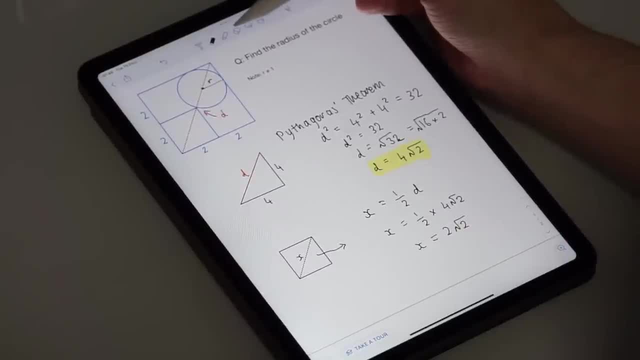 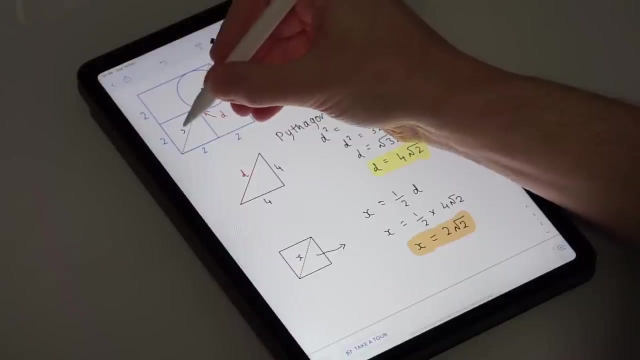 So 2 root 2.. Very nice, So there's our second sort of helpful number that we've worked out, just with a little sort of manipulation of values in our diagram. So let's label on x as this diagonal there. So we have x, we have d. 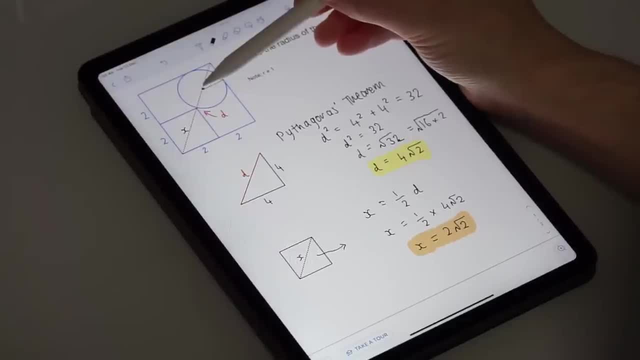 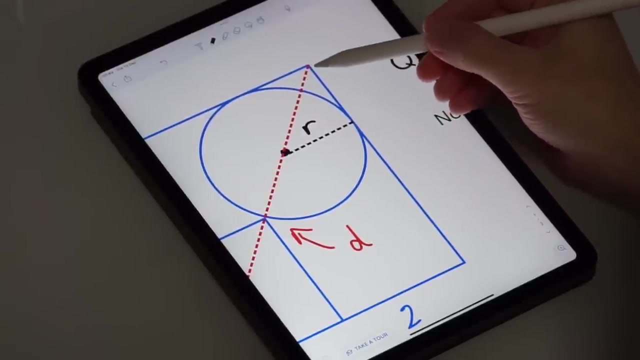 Let's try and work out from here to all the way in the top corner, because this actually isn't the radius, as it has this little sort of extra portion, as you can see This tiny little extra portion here. How can we add that on? 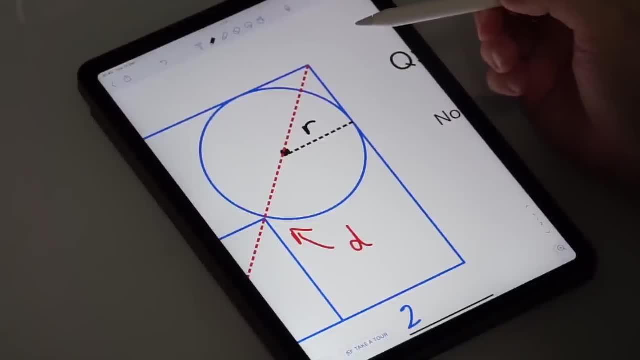 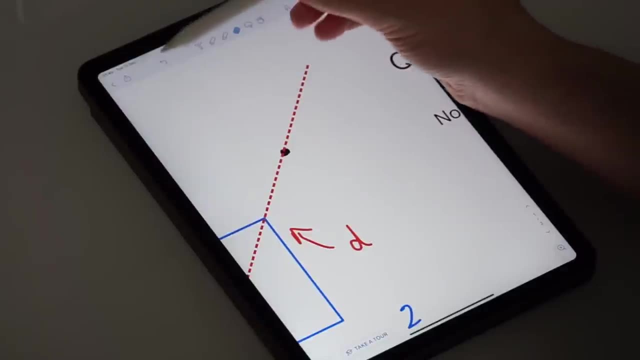 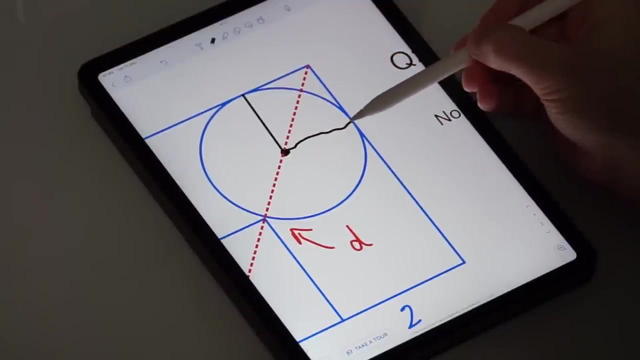 Well, let's look very, very closely at what we're working with here. If I erase a few things here, if we look very closely, I can form another square. That's right, another square in this shape. Take a look at this. 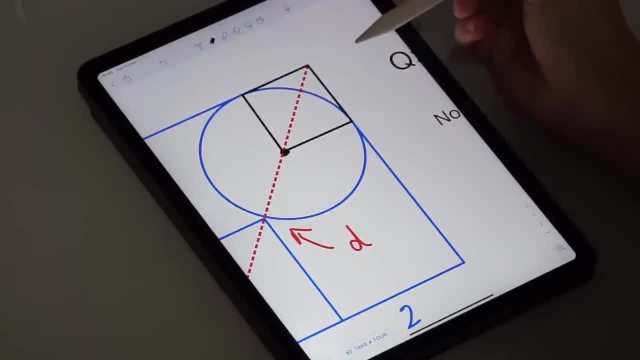 It's like a secret square that we've just drawn And, excuse my stomach, do we know any values of this square? We don't know the diagonal. You might not know what that length is because of this weird extra bit, but you actually do, because look that there is just the radius. 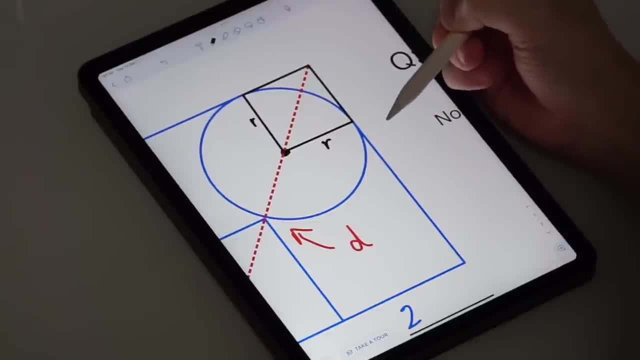 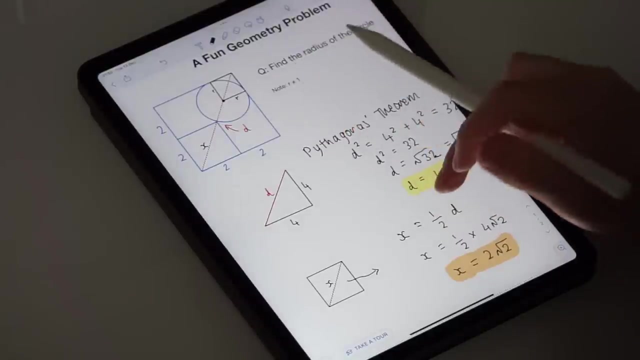 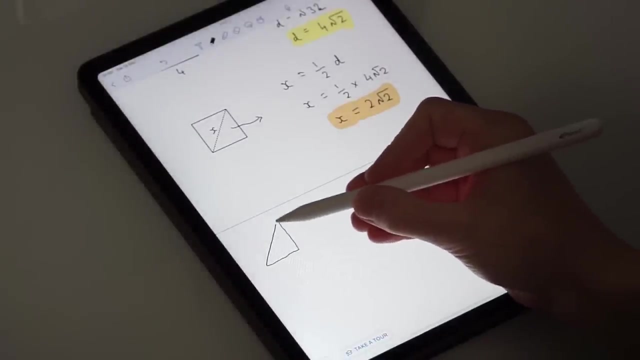 and that there is also just the radius, So this square is r by r. Or we could just take that down here and say: well, we can do a similar thing that we did with this square and turn it into a triangle. Oops, that didn't work. 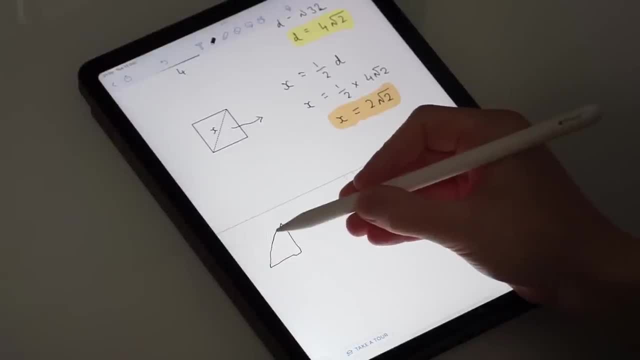 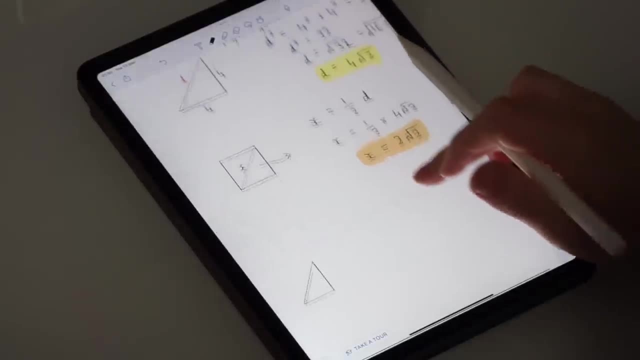 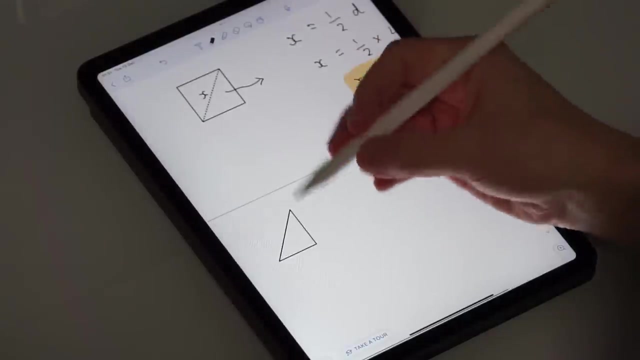 I'm not very good at drawing triangles. apparently, There we go, Can I? Okay Now bear in mind: the reason we could use Pythagoras up here was because it's right angled This time, our triangle in this case, as we saw from before. 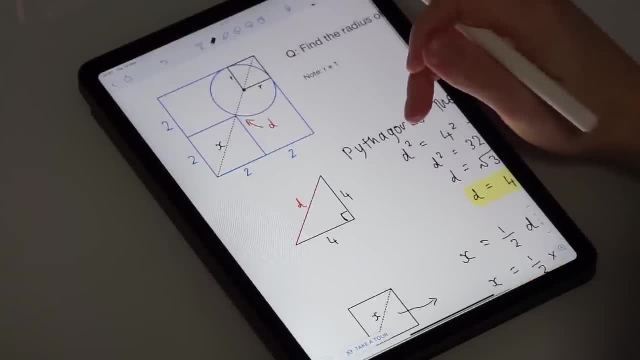 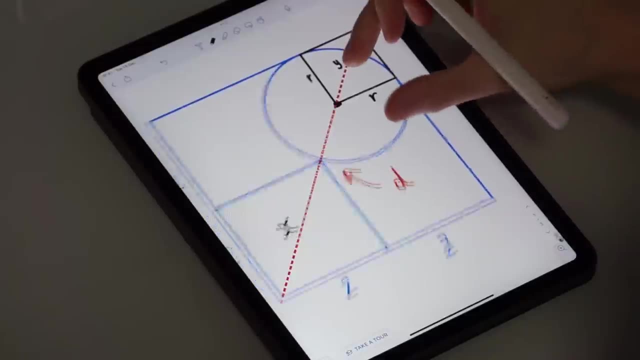 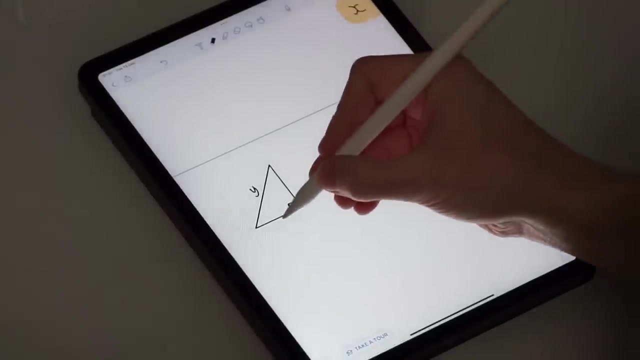 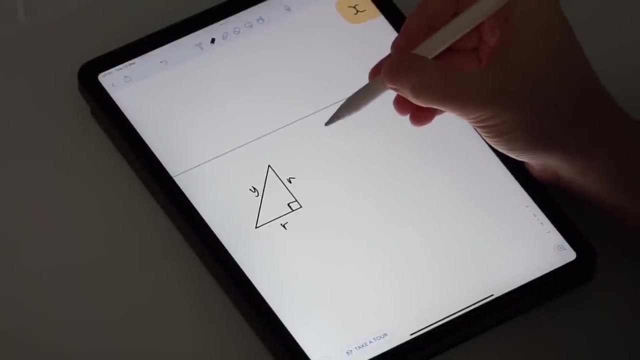 is r by r. So let's call this little diagonal that we're working here, y. Let's work out y. So we have y, then we have r and we have r. Well, using Pythagoras again, y squared is equal to r squared plus r squared. 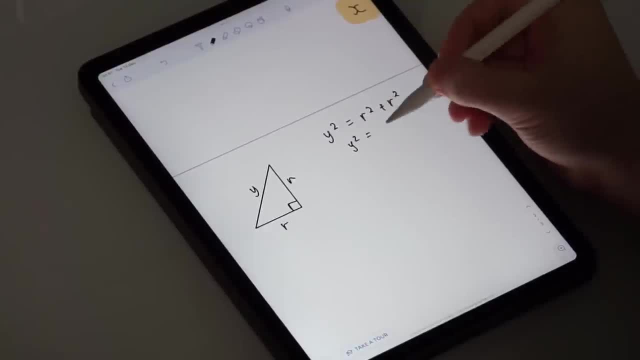 which is just 2r squared, Correct. Let's simplify. If we take the square root of both sides, well, square root of 2r squared. well, the square root of r squared is easily just r, But the square root of 2 is not so easy. 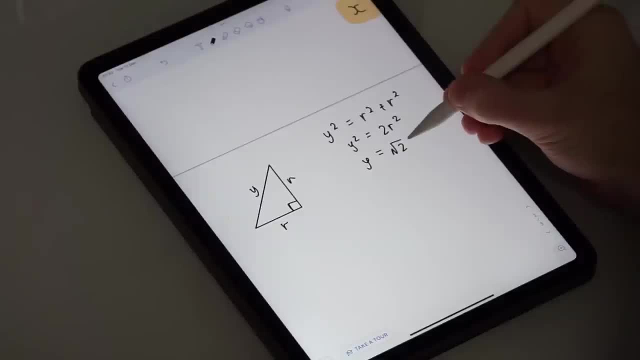 We're going to have a leaf as this: Square root of 2.. Square root of 2 multiplied by r. But this is actually useful for us because it seems pretty familiar, doesn't it? We have a few square root 2s that we have used. 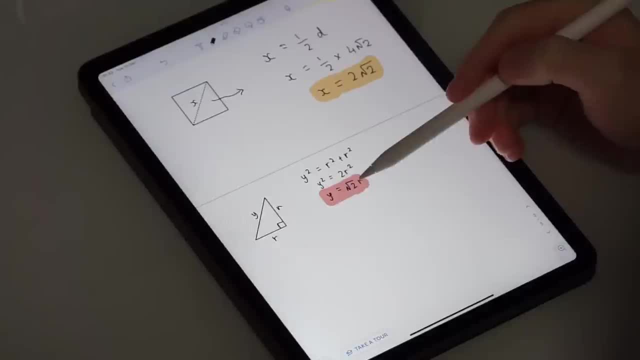 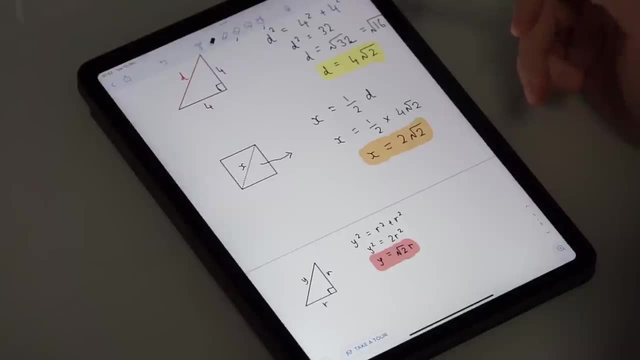 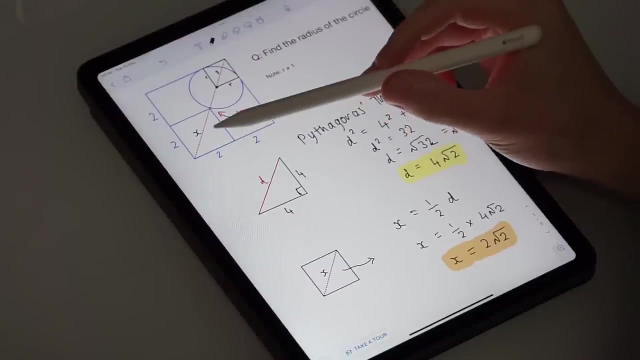 throughout this problem. We have one here, we have one here, we have one right up with the big diagonal we first worked with And, if we remember, we said that this big diagonal is x plus y plus the radius. Well, let's write that down as a big equation. 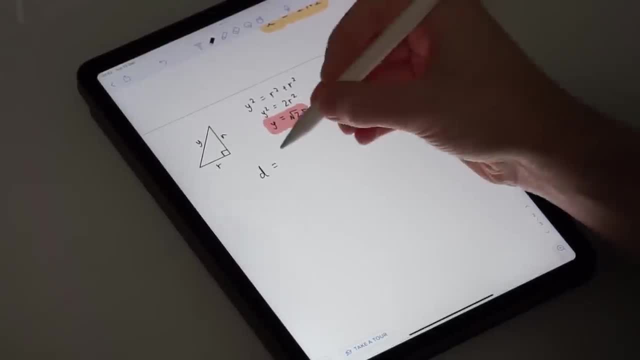 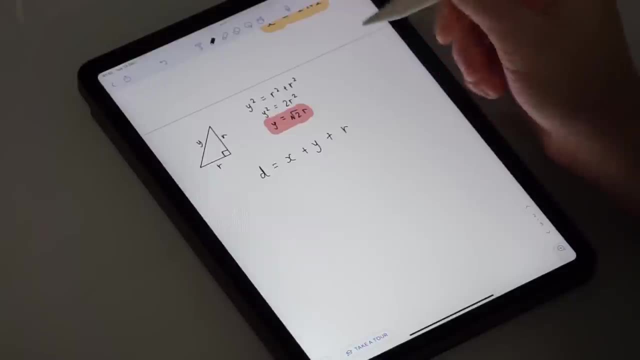 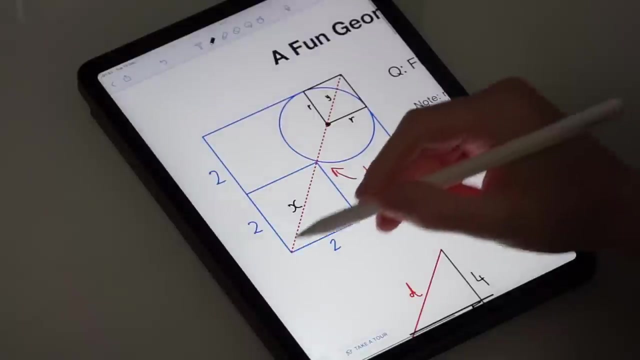 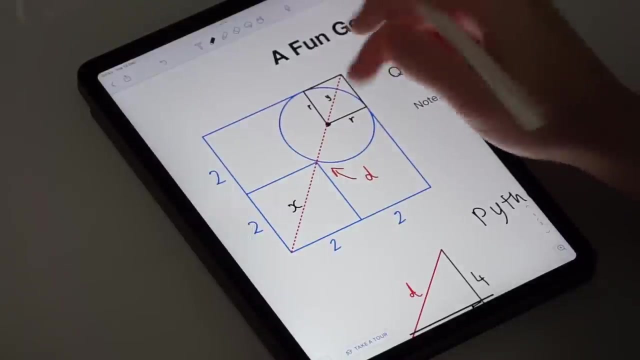 The big diagonal is equal to x plus y plus the radius, And I'll show you that again, just in case that confuses you. We have our big diagonal, We have x, which is from there to there, We have y, which is from here to here. 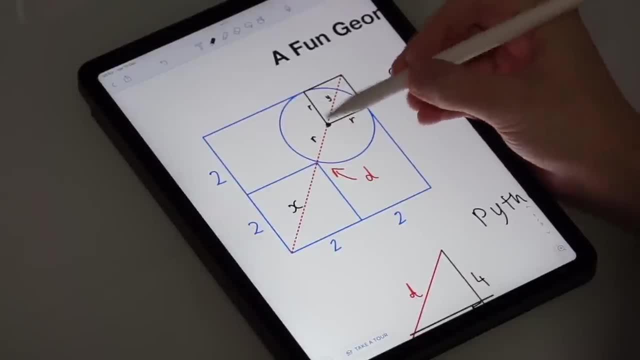 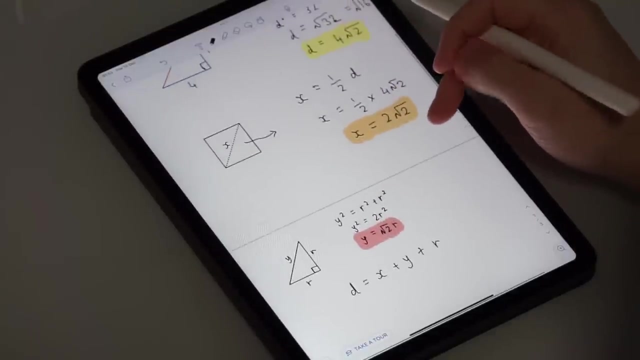 And then we have the radius, which is from here to here, like we said at the start. So let's input all those values that we've worked out. Well, we worked out that our big diagonal d was 4 root 2,. 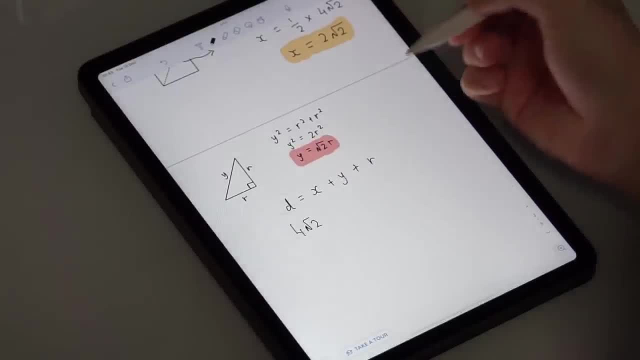 so we'll pop in 4, root 2.. By the way, I've been trying to improve my handwriting. It's actually quite good my handwriting, I'd like to say It's just it's difficult to do on an iPad. 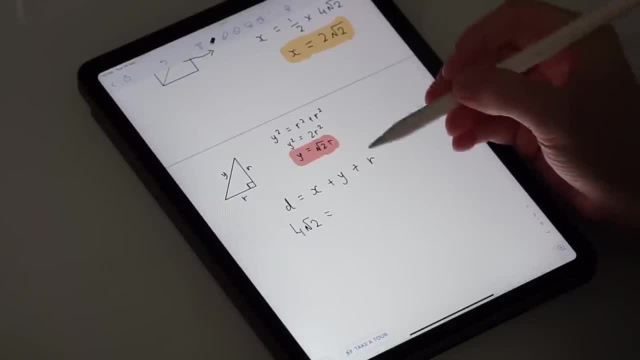 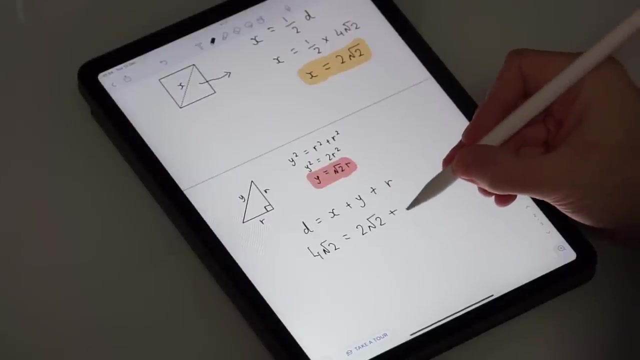 For x, we said it was 2 root 2.. Plus y: What was our y? Oh, it's right there- Root 2 r. And then we add that extra r on the end. Now this just becomes a simple algebraic equation. 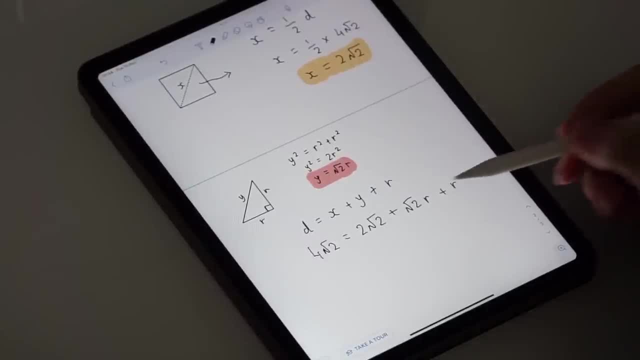 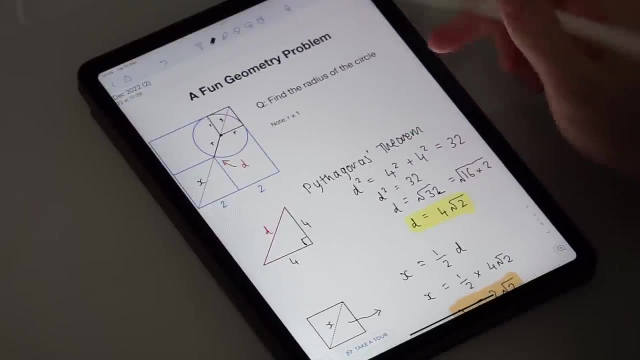 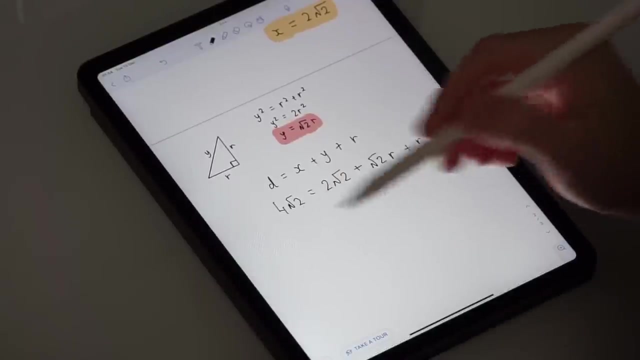 where we must solve for an unknown which, in our case, is r. And don't forget, r stands for radius, which is what the question is asking us in the first place. So let's well take all the numbers to one side. 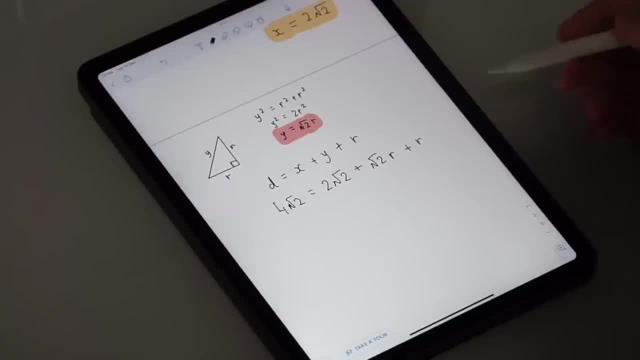 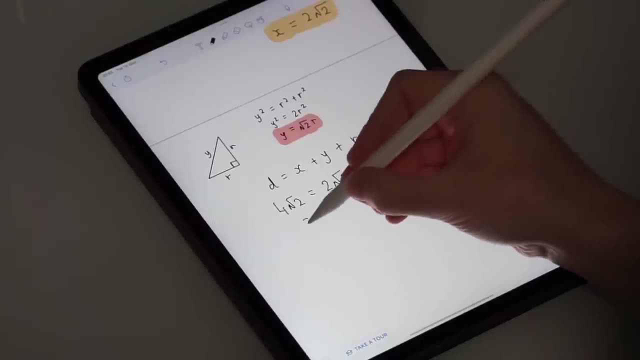 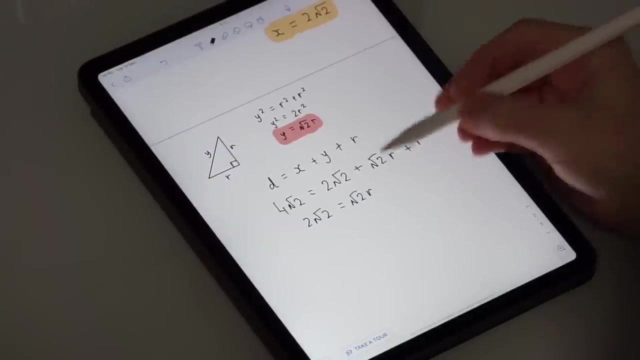 and all the dependent variables to the other. So if we subtract 2 root 2 from both sides of the equation, we'll get 2 root 2 is equal to root 2 r Plus r. And then on this right hand side, 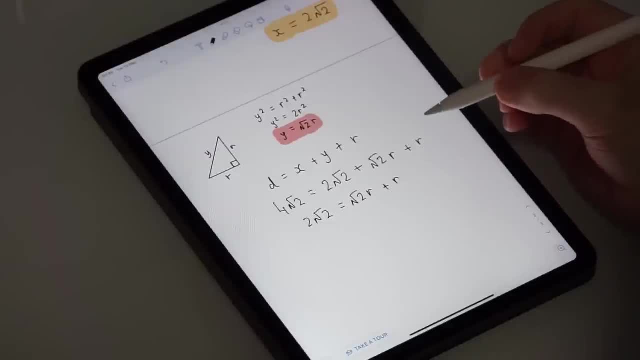 we can factor out the variable r, So we have 2. root 2 is equal to r multiplied by root 2, and then plus 1, because this r is multiplied by 1, as you can see, There's like a sneaky little. 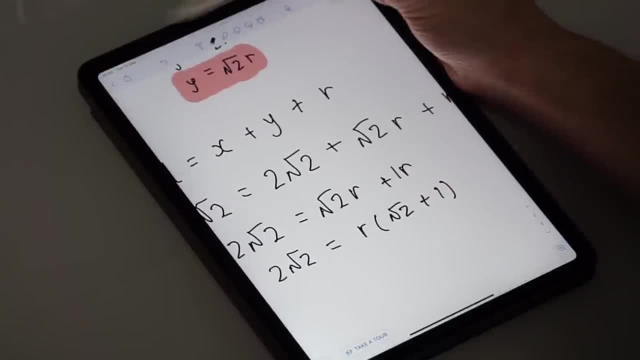 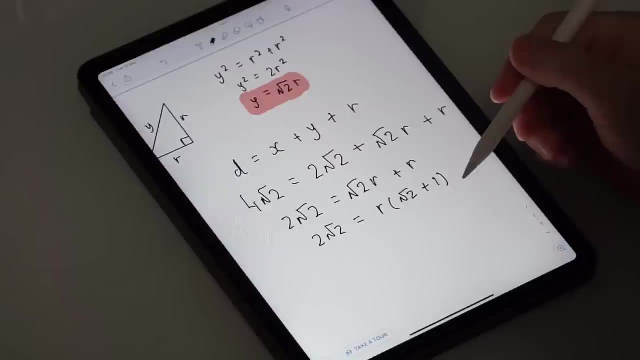 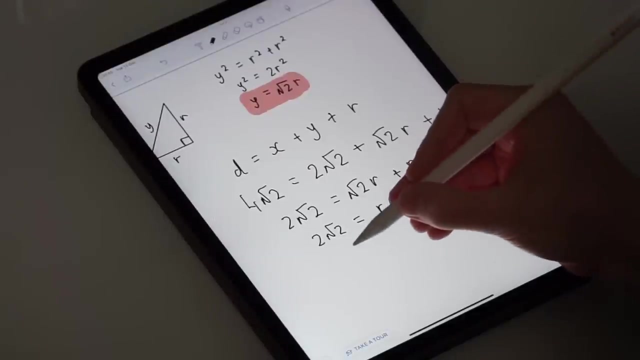 sneaky little 1 in front of there. So now we have this. All that's left for us to do is divide both sides by root 2 plus 1.. And we are left with r is equal to 2 root 2 divided by. 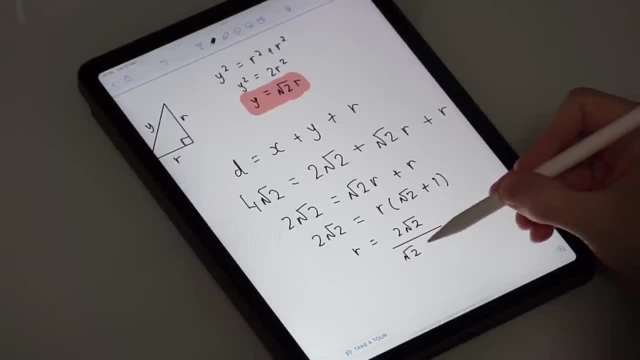 root 2 plus 1.. And we'll pop a nice big box. Dang, it didn't recognise my box. We'll put a nice. in fact, we'll use blue, like the question gave us Around that. there that is indeed. 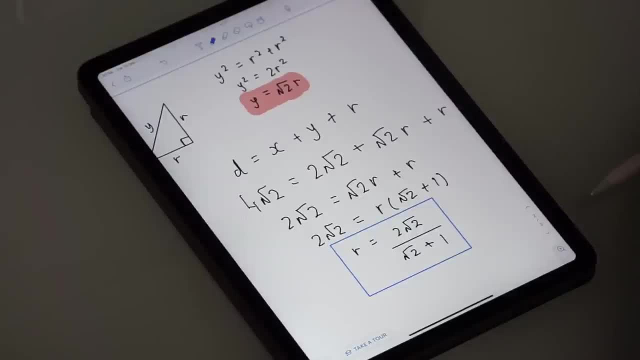 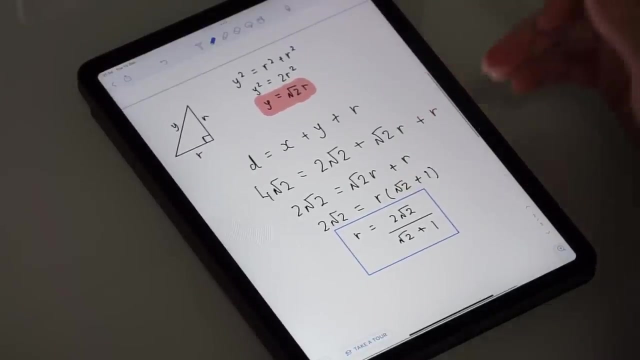 our final answer of the radius: No units, Just nice. A nice third fraction, shall we say. Not so nice, but it's still the answer And it's a very fun, slightly challenging at first, but when you break it down, 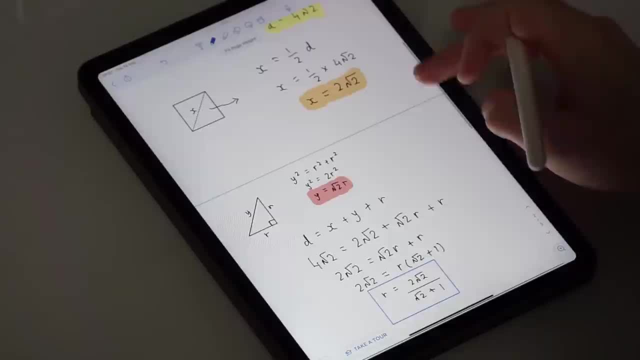 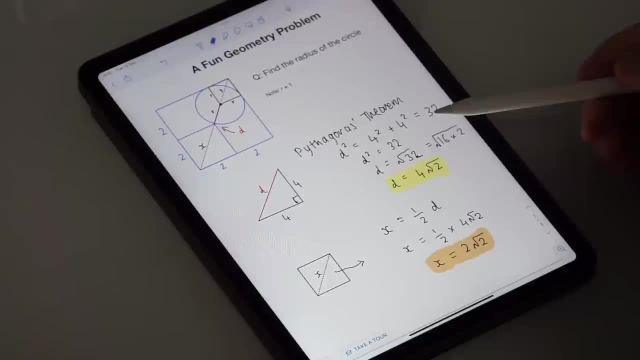 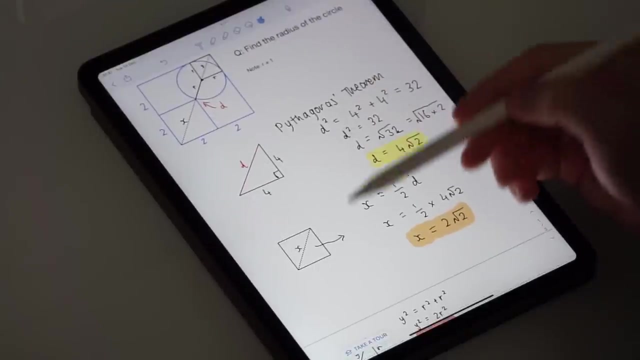 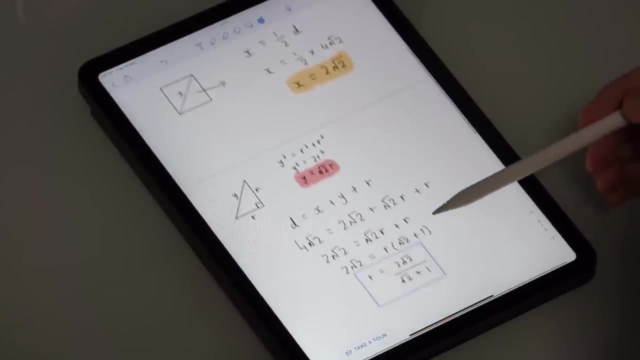 quite simple process to work out. You know you use areas of geometry and algebra together to work out values of triangles, squares. you know simplification methods and substitution And it's all quite a nice problem. that, I think, is very, very fun. 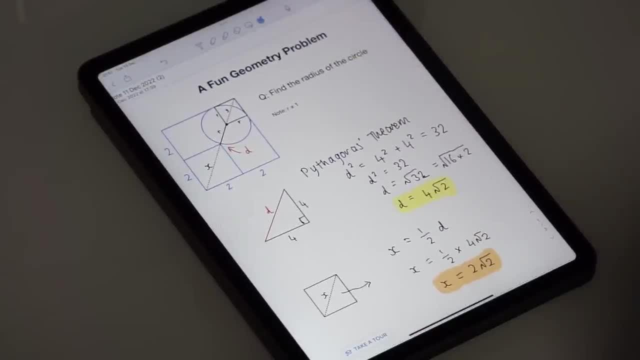 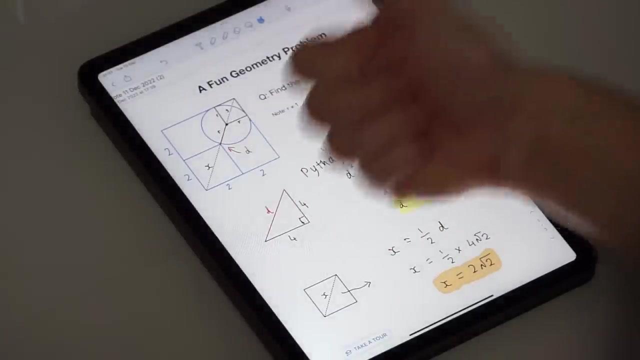 And hence the title, And so I really hope that you all did enjoy. If you did enjoy this video, why not consider dropping it a big thumbs up? It would really mean a lot to me And I'd really appreciate it if you drop some feedback down below. 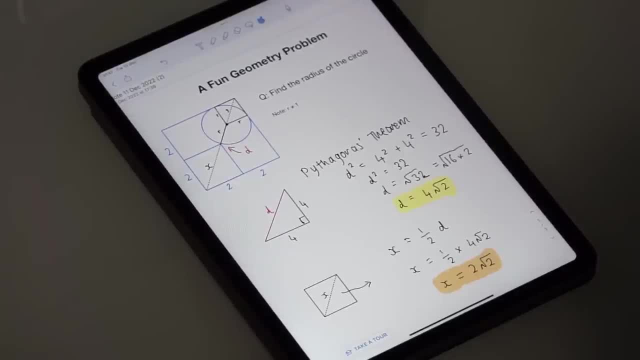 As I said, this is my second ever video here on the channel And I'm having a lot of fun with working with this iPad and making different styled videos for you. In the last video I did lots of different problems. In this one I just did one. 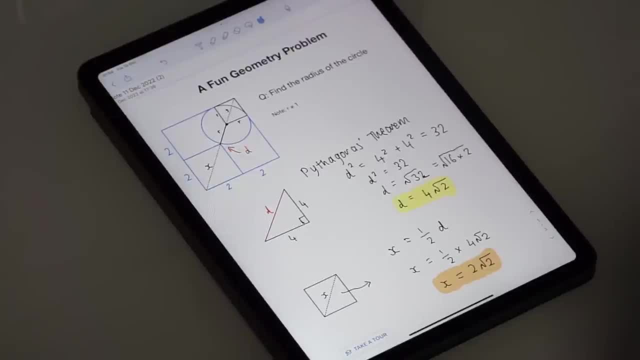 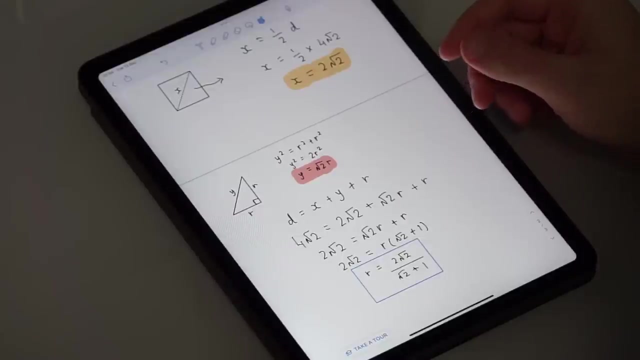 sort of lengthy problem And I'm thinking maybe moving on to sort of more teaching, Because I know I kind of mixed and matched between teaching areas and going through the problem here. But I think it would be good to get a video where I kind of just 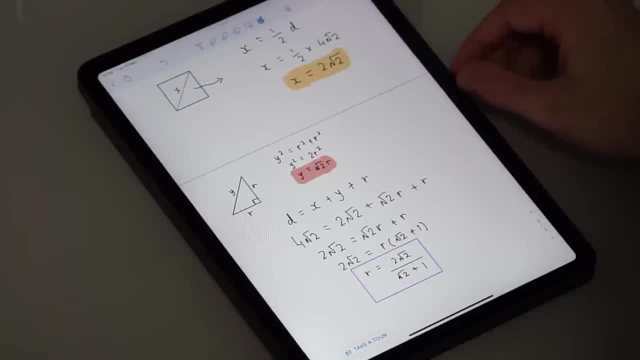 teach a specific area, So I think I might do that in the next one. Let me know what you all think about that. But yeah, thank you all so much for watching. I hope you all enjoyed this problem. Sleep well, Keep studying your maths. 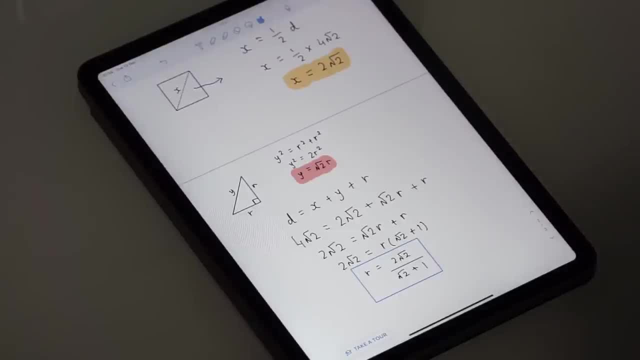 And goodnight everybody, Goodnight everybody.